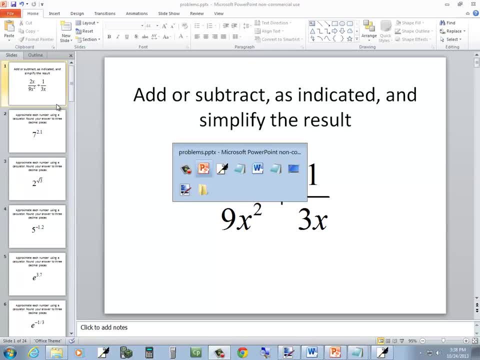 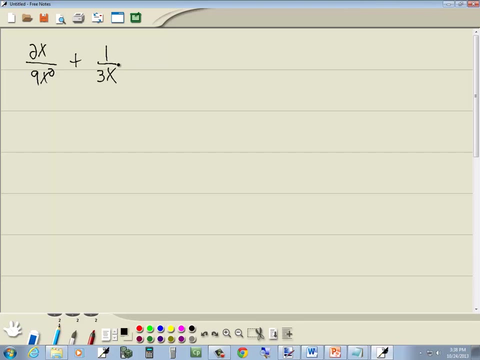 Let's take a look at this problem. We've got 2x over 9x squared, plus 1 over 3x. Now this one's got a little bit of a shortcut. I'm going to ignore it. Do you see it? Fantastic. 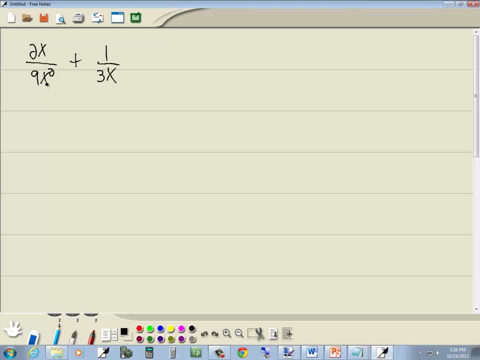 Now our steps say to factor all of our denominators when you have different denominators. I'm actually going to show that here because I want to demonstrate the idea. So 9 is 3 times 3 and x squared is x times x, plus 1 over 3x. Now, after you factor your denominators, then you want to figure out what your LCD is your least common denominator and rewrite each fraction with that new denominator. 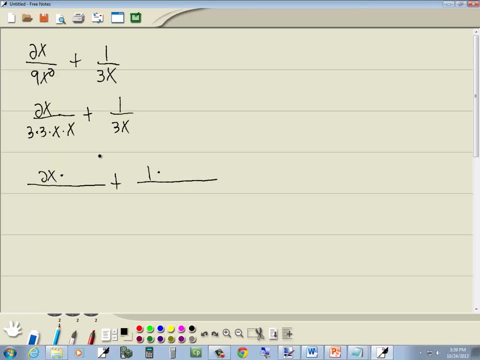 Okay, let's start with the 3s. We're looking for the greatest number of 3s in a single denominator. There's 2 of them here. There's 1 of them here. So the greatest number of 3s in a single denominator is 2 of them right here. 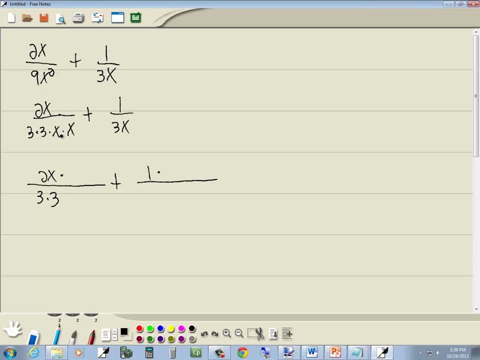 Now we'll go to our next factor, the x. I'm looking for the greatest number of x's in a single denominator. There's 2 of them here. There's 1 of them here. So the greatest number of x's in a single denominator is 2.. 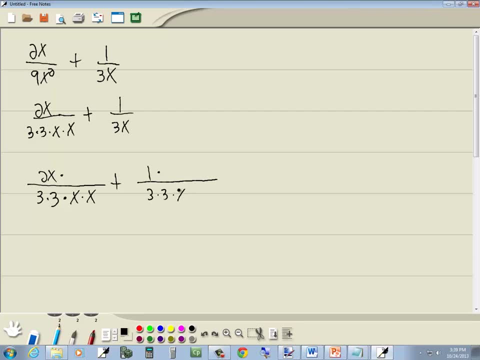 So that's our LCD. Okay, Now, we had a 3 here. We still have a 3.. We had a 3 here, We still have a 3.. We have x, x, x and x. 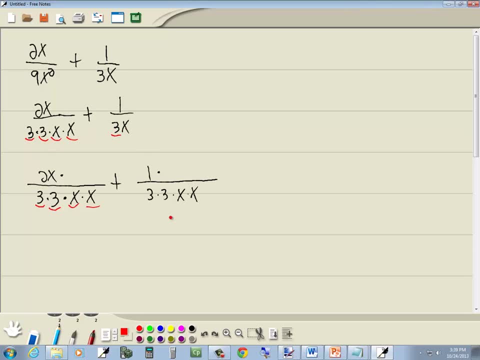 So all those are still there Now. here we had a 3.. Here we have a 3.. Here we have an x. Here we have an x. The two new items down below are this extra 3 and this extra x. 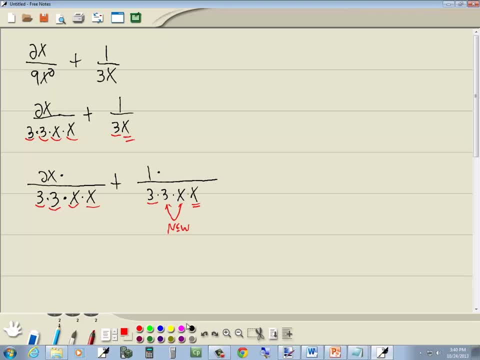 So those are our new items. So whatever new item you put down below here you have to put up on top. So we'll put a 3 and we'll put an x up here. So again, whatever new item you put down here you have to put up on top. 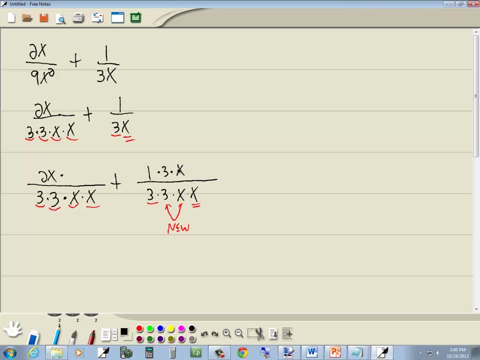 The mathematical rule behind that is: wherever you multiply by the bottom, you have to multiply by the top. That's it, Okay. So that gives us: 2x 3 times 3 is 9 and x times x is x squared.